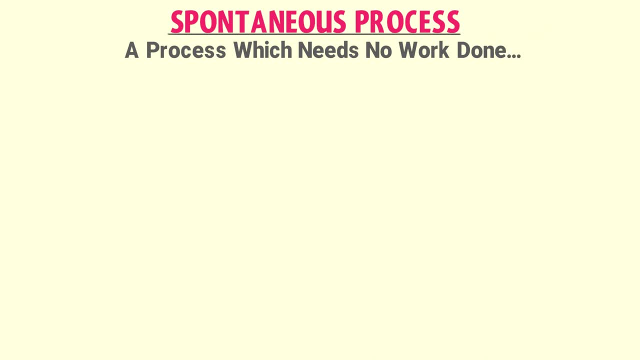 Spontaneous process is a process which needs no energy or work, Or you can say that it is a natural process. For example, diffusion In diffusion, gas molecules move from higher concentration region to lower concentration region without any external aid or external work. 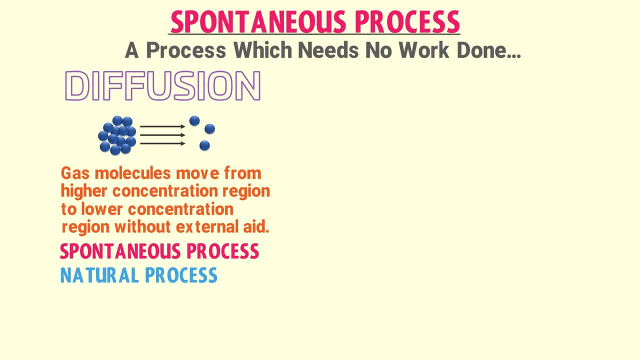 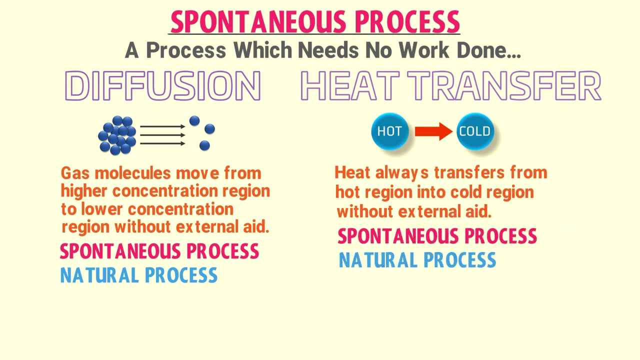 Hence, diffusion is a spontaneous process or natural process? Secondly, heat. We know that heat always transfers from hot body and to cold body without any external aid or external work. Thus, heat transfer is a spontaneous process or natural process? Let me ask you a very important question. 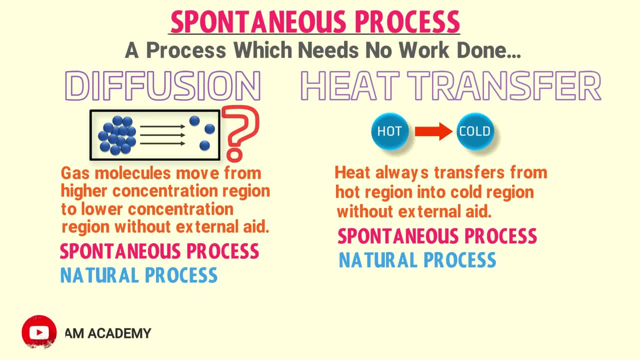 Why gas molecules move from higher concentration region to lower concentration region? Your answer will be, Sir, it is a spontaneous process or natural process. It is nature which forces all the molecules to move from higher concentration region to lower concentration region. Secondly, if I ask you why heat Q always move from hot objects towards cold objects? 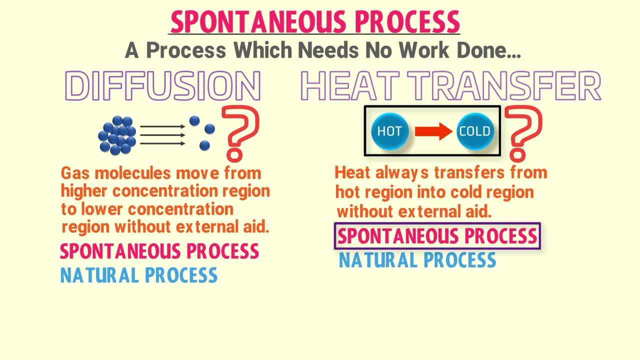 Your answer will be: Sir it is a spontaneous process or natural process. Sir it is a spontaneous process or natural process. Sir it is a spontaneous process or natural process, It is a spontaneous process or natural process. It is nature which provides energy or forces heat Q to move from hot objects to cold objects. 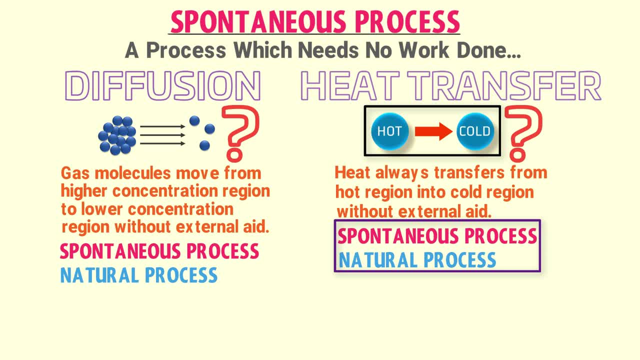 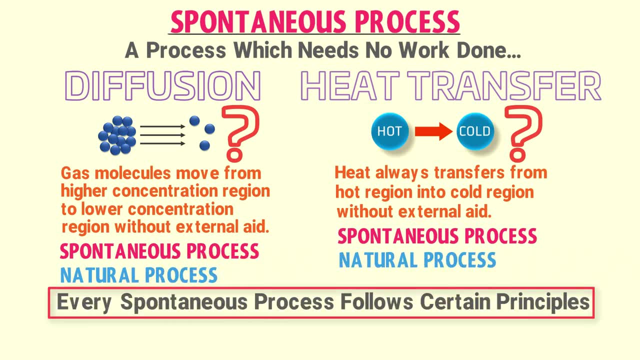 Now here is one very, very important point which, believe me, a lot of people miss it. The point is that every spontaneous process or natural process follows certain principles. Let me repeat this important statement: Every spontaneous or natural process follows certain principles. For example, gas molecules only flow if they are large in number in one region and small in number in other region. 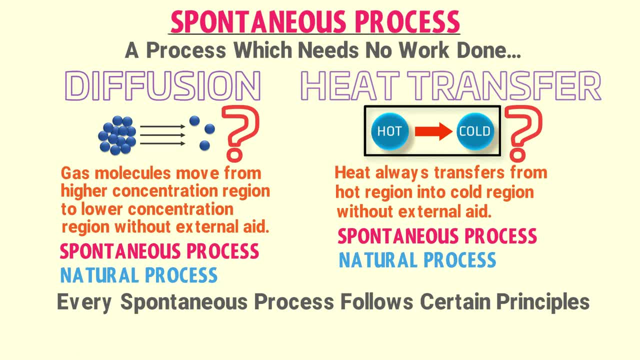 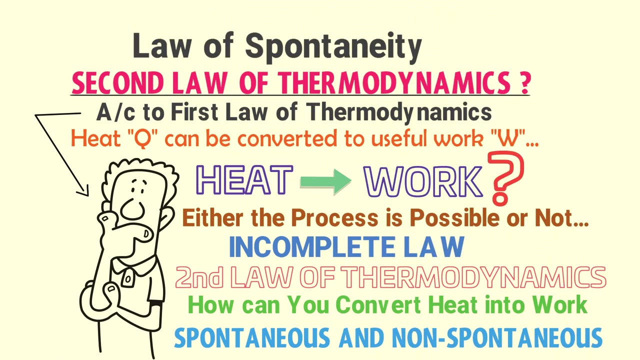 Secondly, heat only transfers from one object to another object if there is temperature difference. Therefore I say that every natural process or spontaneous process follows certain principles. Without them, no spontaneous process or natural process can occur. Here remember this very famous MCQs, that second law of thermodynamics is also known as a law of spontaneity. 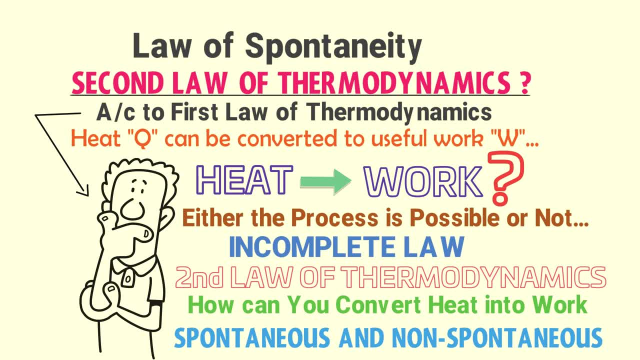 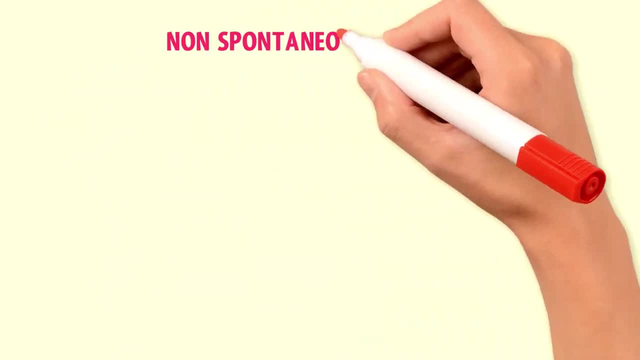 It means that second law of thermodynamics is a natural. Why I call second law of thermodynamics as law of spontaneity, a natural law? Wait, I will teach you this later. Now, what is non-spontaneous process? Let's consider an object present on surface of the earth. 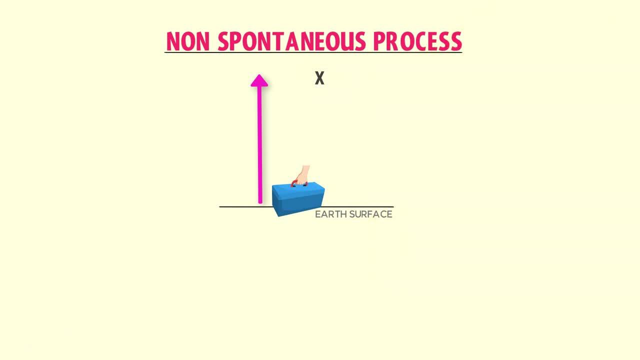 You want to rise this object to point X. Does this object rise to point X by itself? The answer is absolute: no, You do so. You have to do some sort of work on this object to rise it to point X. Hence, objects do not rise above the surface of the earth by themselves. 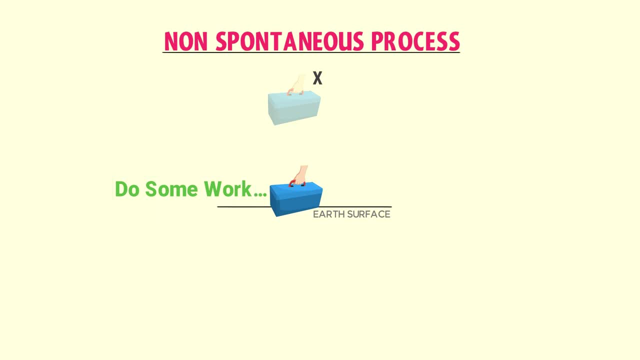 We have to do some sort of work on them. Thus, rising an object above the earth's surface is a non-spontaneous process. You and I need to do some sort of work to proceed. a non-spontaneous process, Remember that. 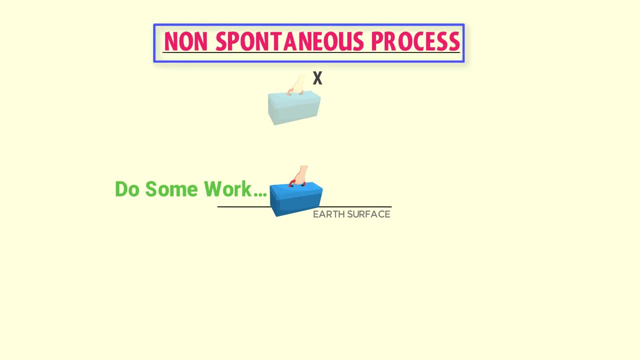 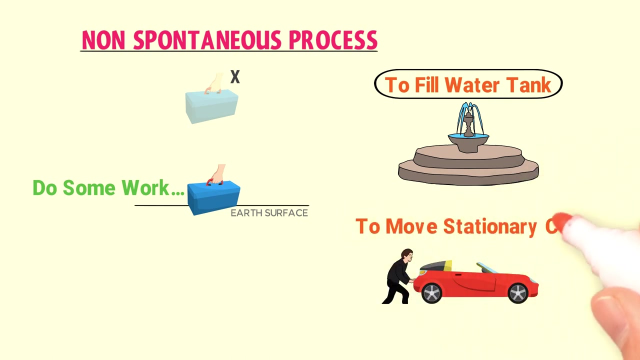 A non-spontaneous process always needs some sort of energy or work to be proceed further. Other examples of non-spontaneous process are to fill water tank at a certain height. The another example is to move a stationary object. These are all the examples of non-spontaneous process. 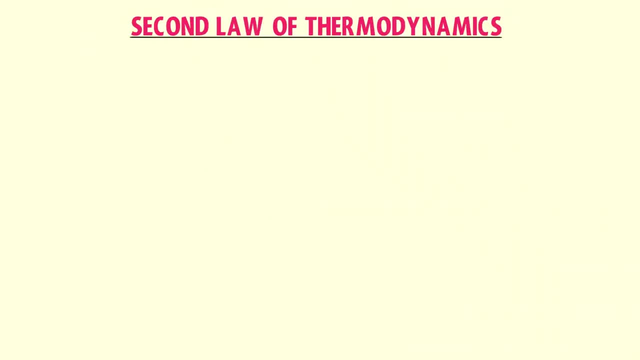 Now let me teach you second law of thermodynamics. Remember that If you learn the working of heat engine, you will easily learn second law of thermodynamics. Let's consider a hot reservoir and a cold reservoir. Let the hot reservoir is at temperature T1 and the cold reservoir is at temperature T2.. 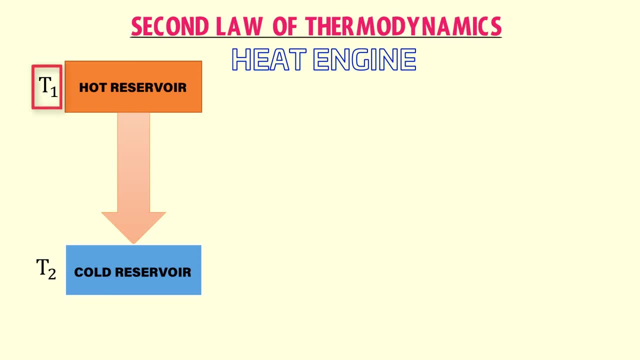 We know that temperature T1 is greater than temperature T2.. Thus, heat transfer will occur between them, This hot reservoir and cold reservoir, due to temperature difference. If I ask you why heat transfers from hot reservoir to cold reservoir, Can you answer this question? 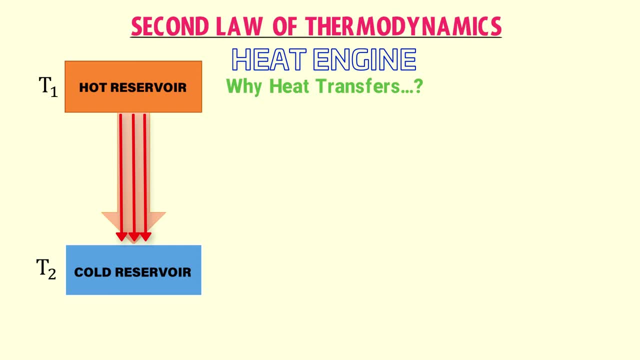 Well, your answer will be, sir, this heat transfer is a natural process or spontaneous process. I will say: okay, Now what will happen if I remove this cold reservoir? Will heat transfer occur? You will say no, sir. 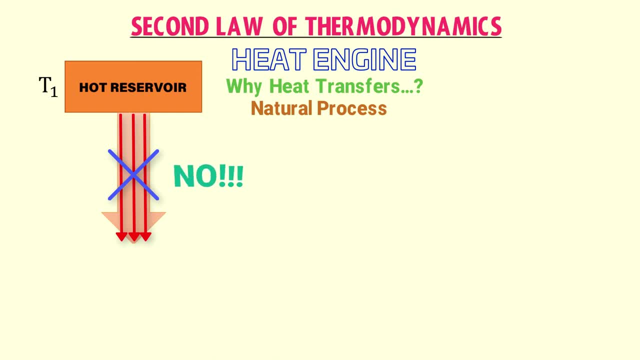 Because heat transfer only occurs when there is hot reservoir and cold reservoir, Or if there is temperature difference. Therefore, the first point we learn in this example is that heat transfer will only occur when there is hot reservoir and a cold reservoir. Remember that hot reservoir is also known as a source and cold reservoir is also known as a sink. 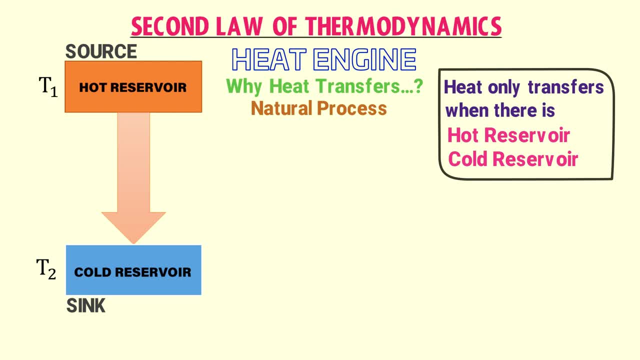 Now let's consider that hot reservoir, a source at temperature T1, loses heat Q1. We construct an engine between this hot reservoir and cold reservoir. Now this heat Q1 enters to the engine, Engine will convert a part of this heat Q1.. 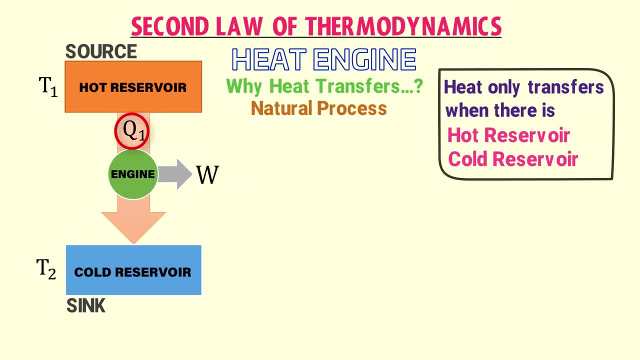 And to useful work. W And engine will reject or expel a part of heat Q1 to the sink or cold reservoir. Let me simplify it further. When engine absorbs this heat Q1 from the hot reservoir, a source it divides, 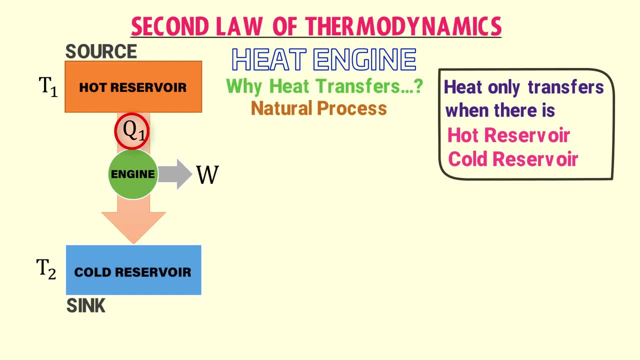 Means the engine divides the heat into two parts. Engine converts one part of heat- Q1. To useful work- W, And engine expels a part of heat Q1 and to cold reservoir, a sink, as heat Q2.. Thus we can write: heat Q1 absorbed by the engine from hot reservoir is Q1 is equal to Q2 plus W. 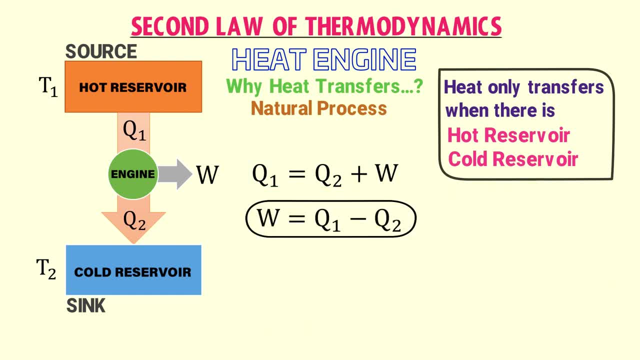 Now rearranging this equation, we get: W is equal to Q1 minus Q2.. Thus, from this heat engine, we learned two very important points. Firstly, it teaches us that heat transfer requires hot reservoir- a source, and cold reservoir, a sink. 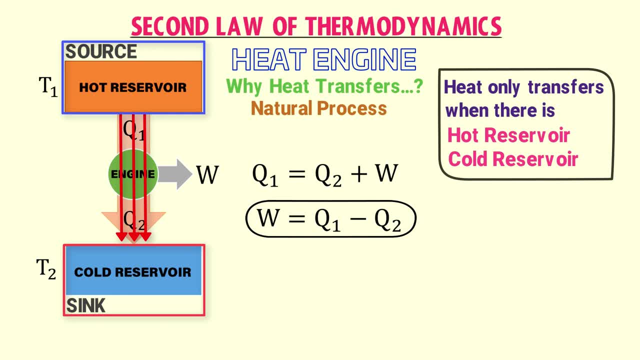 If there is no cold reservoir, a sink, heat will not transfer from hot reservoir a source. Secondly, all heat cannot be converted to useful work. For example, when engine absorbed heat Q1 from the source, engine doesn't convert all heat Q1 to useful work W. 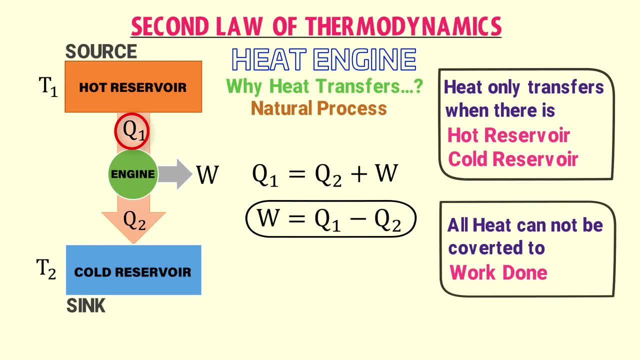 Rather engine wastes or expels heat Q to the sink or to the cold reservoir. Therefore I say that all heat cannot be converted to work. If you have learned all these basic concepts, I congratulate you. You have already learned the second law of thermodynamics. 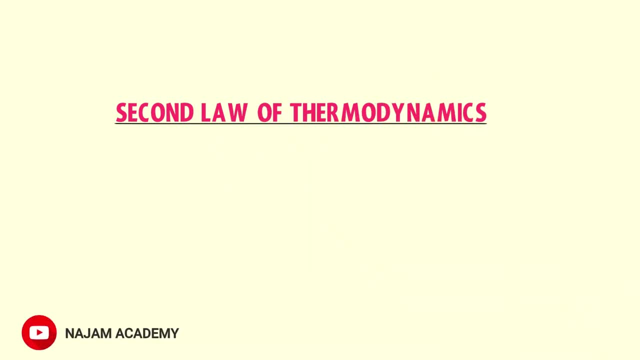 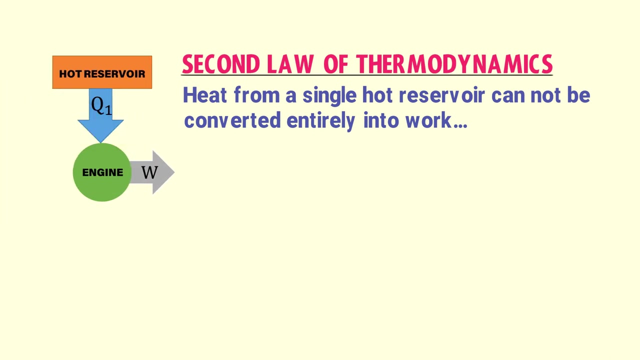 Second law of thermodynamics. Lord Kelvin defines second law of thermodynamics as heat from a single or from a hot reservoir cannot be converted entirely and to work done W It means engine cannot absorb directly the heat of hot reservoir. When engine doesn't absorb the heat of hot, 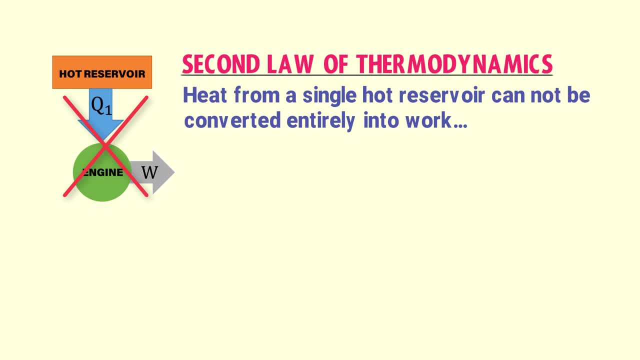 reservoir, a source, then how can work be done? Therefore, the second law of thermodynamics teaches us the method: that for engine to absorb heat Q1 from hot reservoir, there must be a cold reservoir, a sink. In the previous slides, 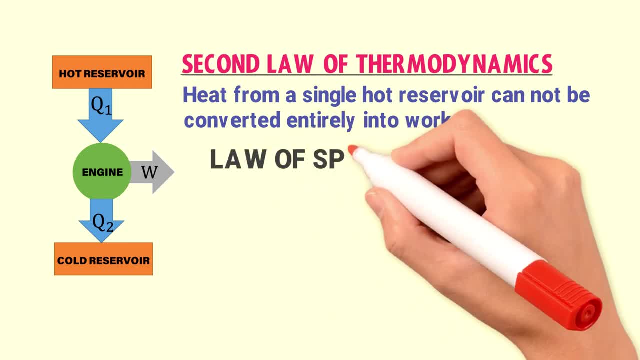 I told you that second law of thermodynamics is also known as a law of spontaneity. It is because heat transfer only occurs when there is source and sink. While second law of thermodynamics also teach us this method are states that you can only utilize the heat Q of a source.